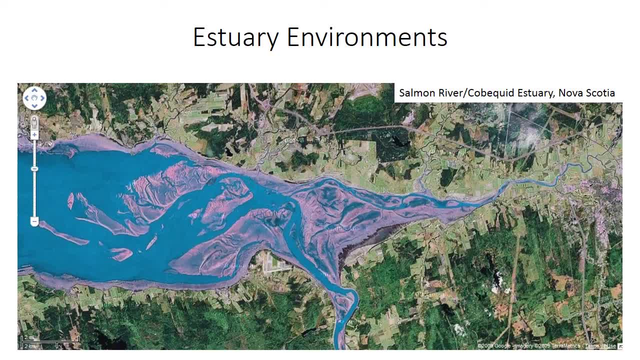 In the previous video you learned about delta environments, one of the depositional settings that forms at the interface between rivers and the ocean. So this video introduces estuary environments, which is another mixed fluvial marine depositional setting. Although both estuaries and deltas form where rivers flow into the ocean, it turns out they have completely 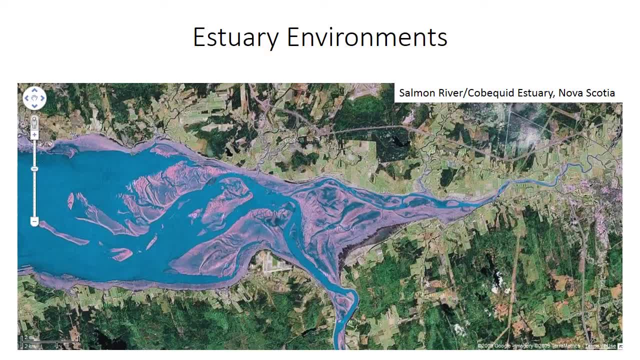 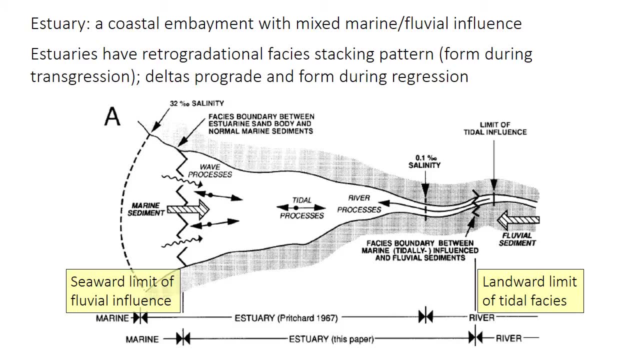 different depositional characteristics and a wide variety of different faces in each setting. Estuaries are coastal embayments with mixed marine and fluvial influences. They're defined as the area between truly marine faces and exclusively fluvial faces, So they have a 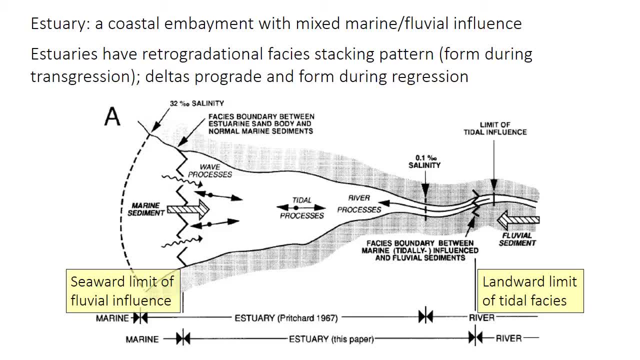 mixture of marine and fluvial influences in their faces. This definition is slightly different from the use of the term estuary that you might encounter in geography or in ecology. In the rock record, estuaries always form during transgression, So they, by definition, have 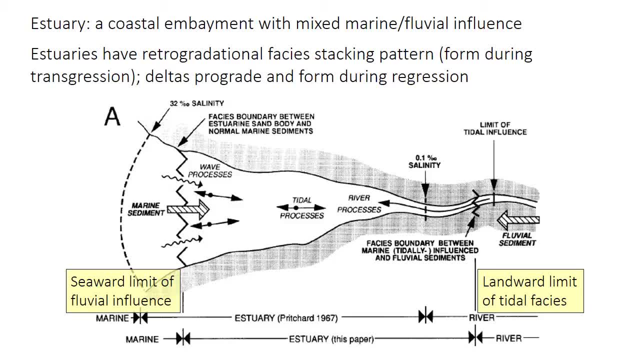 retrogradation and transgression, So they have a mixture of marine and fluvial influences. In contrast, deltas are always progradational. So even though, as we'll see, some deltas and estuaries, particularly tide-dominated deltas and estuaries- look similar, they can be distinguished. 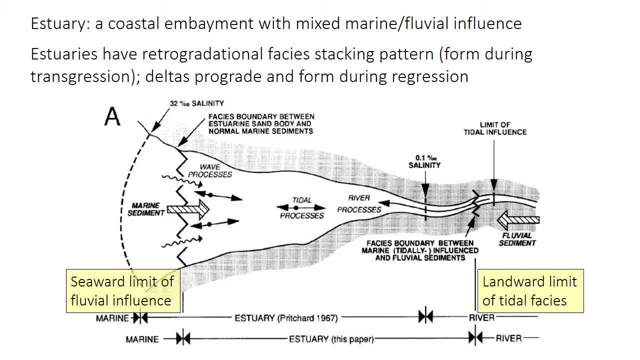 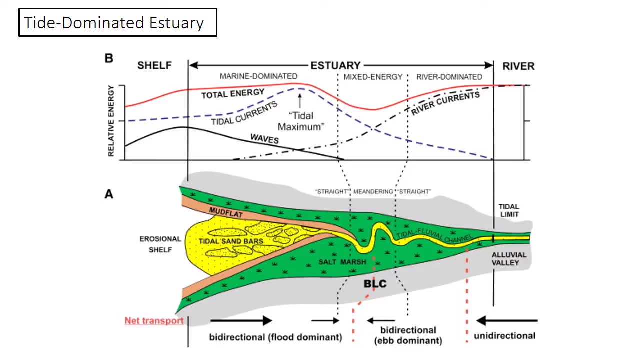 by their facey stacking pattern. Again, the restriction of estuaries to purely transgressive settings may differ from other uses you might find in ecology or in geography. One of the most characteristic features of estuaries is a triploid. A triploid is a three-part division of energy levels Because estuaries have energy supplied. 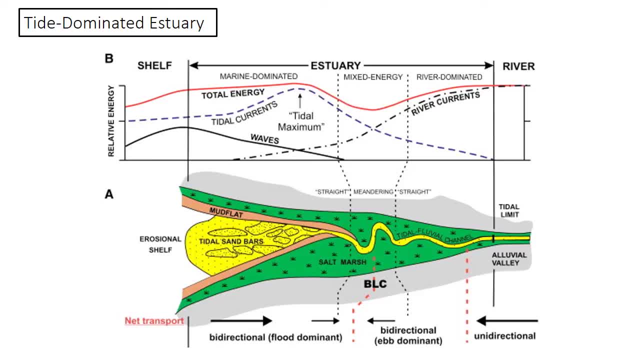 from the ocean side in the form of tides or waves, and from the landward side, from the river. energy levels tend to be lowest in the middle of the estuary and highest at either end. So this diagram here shows a schematic model of a typical tide-dominated estuary: The 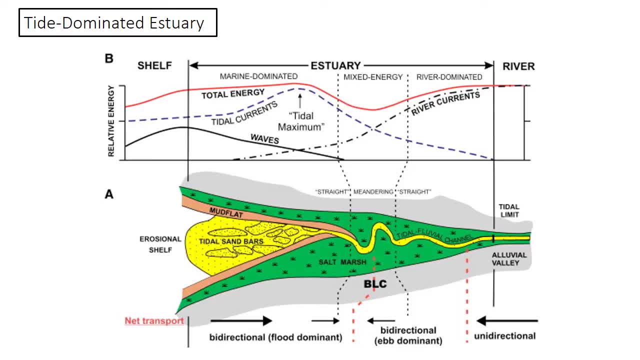 distribution of energy is shown in the upper panel and the environments in the lower panel. I'm not going to spend a lot of time on the sedimentary structures here, because they're very similar to faces you find on tidal flats In the tidal fluvial channel, for example. you'd expect to find flaser bedding lenticular. 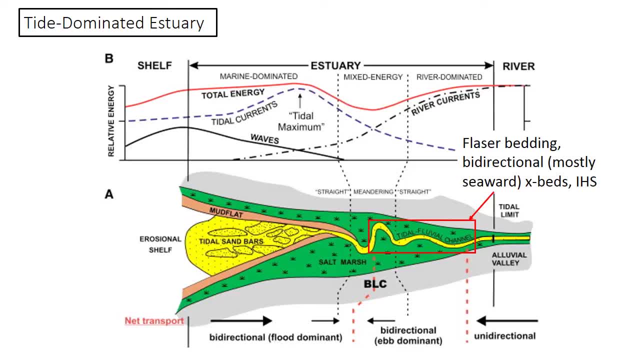 bedding, primarily ebb-dominated or seaward-dominated, crossbedding, perhaps inclined heterolithic stratification, all faces that you heard about in the tidal flats lecture On the ocean side, the tidal sand flat here will be dominated by higher energy herringbone. 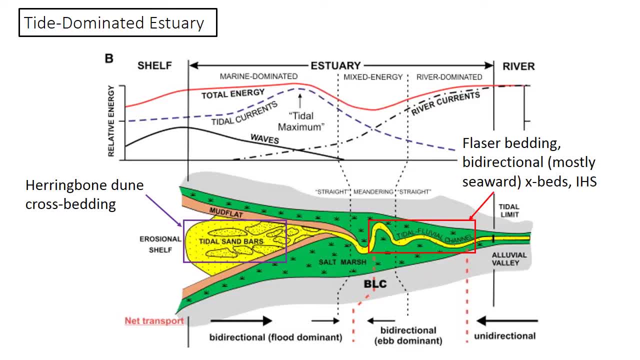 which is bidirectional crossbedding. So if these faces here are the same faces you would find in a tidal flat. how are you going to distinguish the two environments in the rock record? Well, one way is that estuaries have this lower energy central zone and therefore have 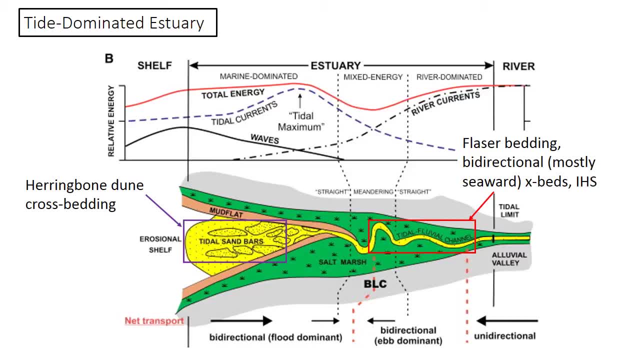 resulting finer grain size and lower energy sediment structures there That you're not going to really find that in a tidal flat. Also note at the very bottom the shift between flood-dominated or landward-directed currents in the outer part of the estuary and the 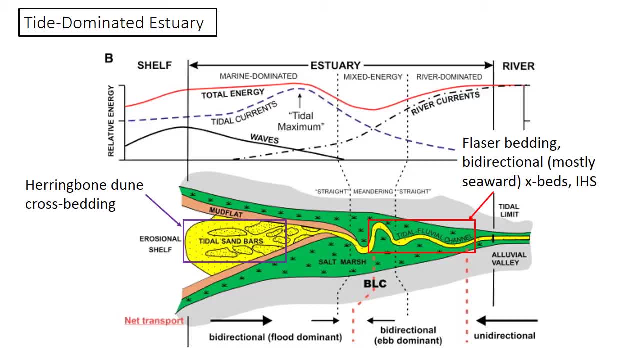 estuary versus ebb-dominated or seaward-directed currents in the inner part. Tidal flats again are not going to have a shift in current direction like that. We'll spend some more time on wave-dominated estuaries because they have some new depositional. 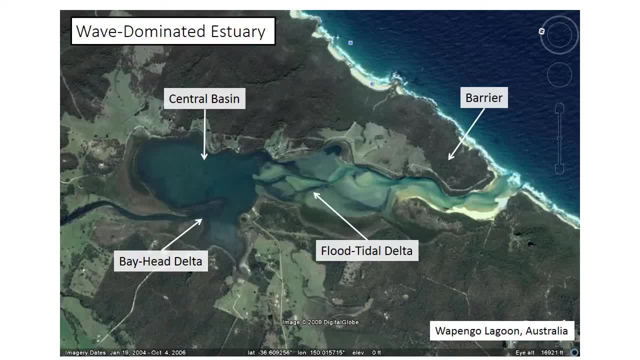 sub-environments like this Bay Head Delta, where the river enters the central basin, the central basin itself, and the flood tidal delta, where the incoming tides enter the central basin. So I'll talk about those settings and their expected facies in a little bit more detail. 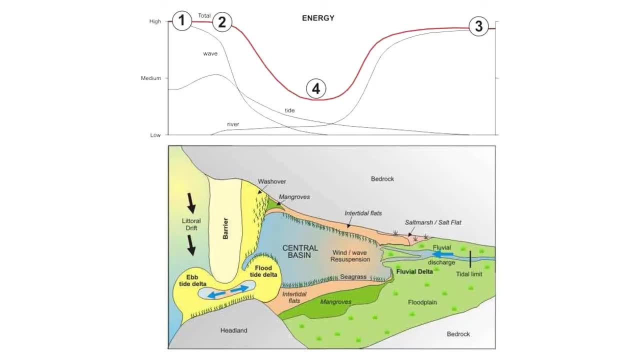 in the next few slides. The tripartite energy regime with a central low-energy area is even more strongly developed in a typical wave-dominated estuary. So, given this distribution of energy levels and sediment transport processes, whether waves or tides or fluvial, you should be able to predict the type of facies and sedimentary. 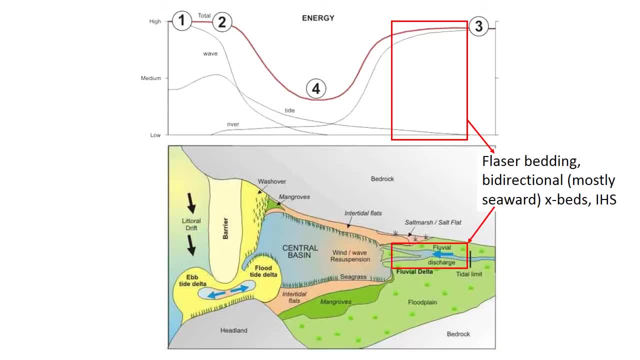 structures you'd expect in each region. For example, again the Tidal flats again are not going to have a shift in current direction like that. Bay Delta, The tidal fluvial-dominated region, has primarily fluvial currents but some tidal influence. 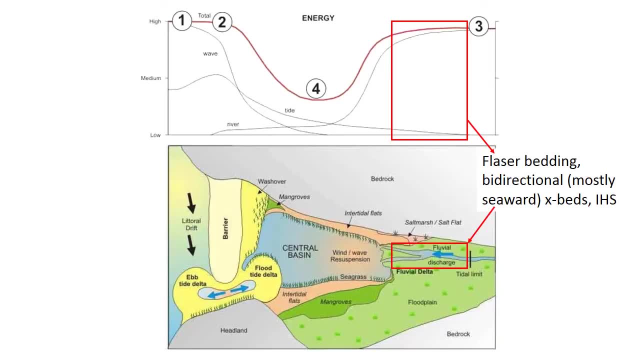 so there would be some bidirectional crossbedding. We've got again flaser bedding, ebb-dominated bidirectional crossbeds, inclined heterolithic stratification on the channel meanders. The low-energy central basin, because of its very low energy levels, will be dominated. 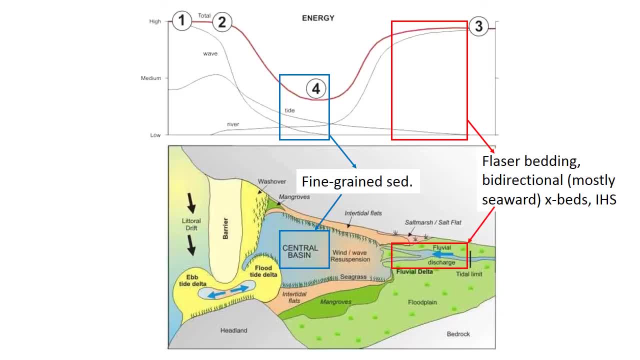 just by fine-grained mudstones or siltstones. typically, The seaword side of the barrier is just a beach, and so it'll contain beach facies, low-angle upper plane bed laminations. if you go offshore, there'll be a shore face and 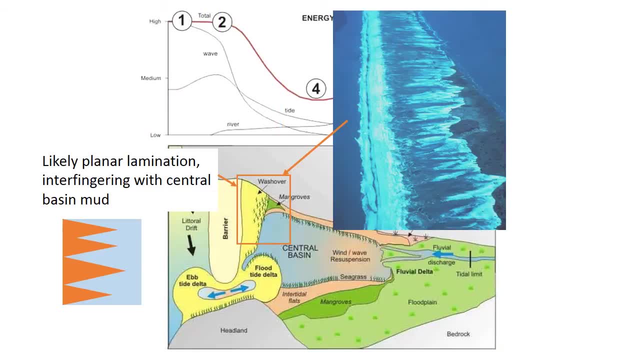 so forth. So a couple new environments. The area here labeled wash-over is dominated by sand supplied in these occasional storm events. You get a big storm, it surges, the big storm surge builds up and it washes over the barrier. So because the sediment here is transported by high-energy storm surge, it'll almost certainly 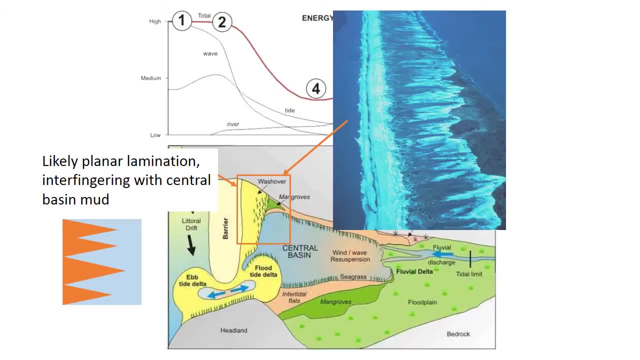 be sand-rich And we'll likely have planar laminations similar to a beach. probably These wash-over lobes will inter-finger with the central basin muds and that just means that the two facies are inter-bedded. 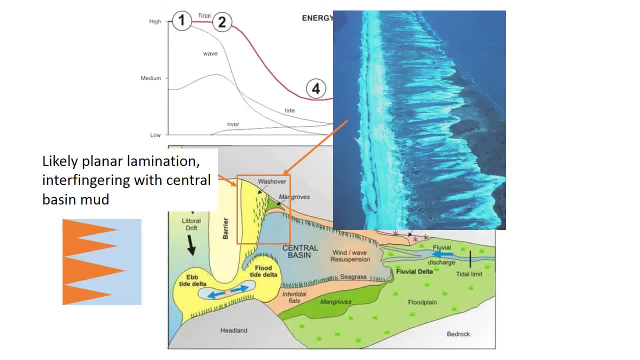 The wash-over will thin towards the land, the central basin will thin towards the ocean. I've kind of illustrated that schematically in the diagram here. the orange wash-over facies thinning towards the land, the blue central basin facies thinning towards the. 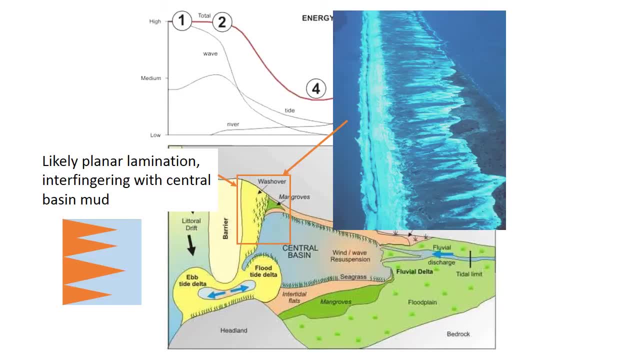 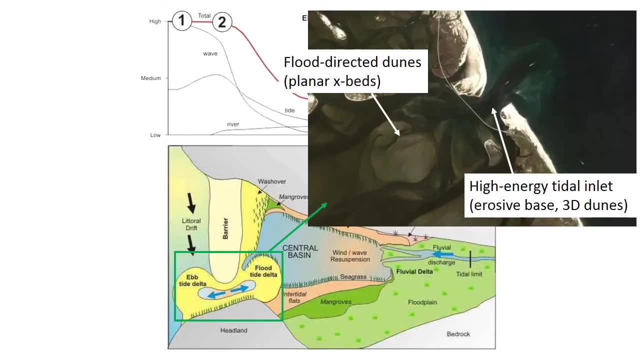 ocean and they're inter-fingered, like you would sort of interlock your fingers with both hands. So the last sub-environment that I'll cover briefly is the tidal inlet region. We'll discuss this sub-environment in more detail in the next lecture, when we talk about 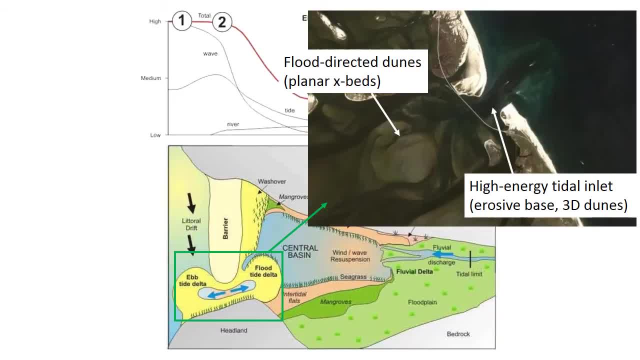 barrier islands. But, briefly at least, it includes a deep and high-energy tidal inlet. Because it's high-energy, it has an erosive base and it has 3D dunes, you know, given the high energy and the coarse grain size in this sort of setting. 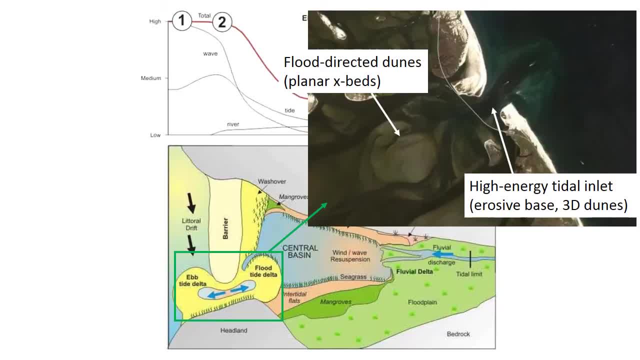 This thing called the flood tidal delta is basically sort of a complex of sandbars. You know, it's kind of like the sandbars that the incoming or flood-directed tidal current builds as that current spreads out and fans out into the central basin. You know, as the current spreads out, it slows down, it deposits sediment, it creates these. 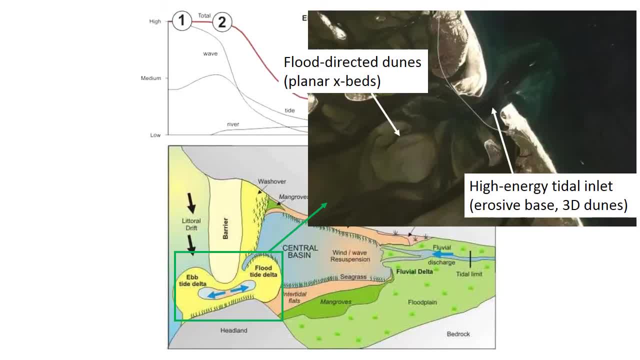 bars that kind of migrate into the bars and dunes that migrate into the central basin. So because of that it's dominated by these large dunes. there's large planar crossbeds, probably some smaller trough crossbeds. we'll talk about the specific patterns of waterflow. 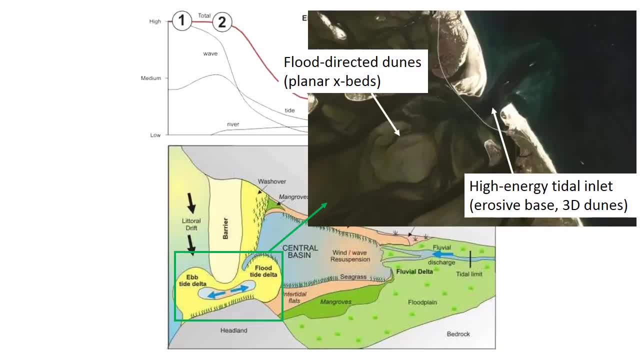 in this setting next time. So there's a lot of components to this wave-dominated estuary. it's a little overwhelming probably, but if you just focus on the energy levels, the sediment transport, you really can predict a lot just from there. 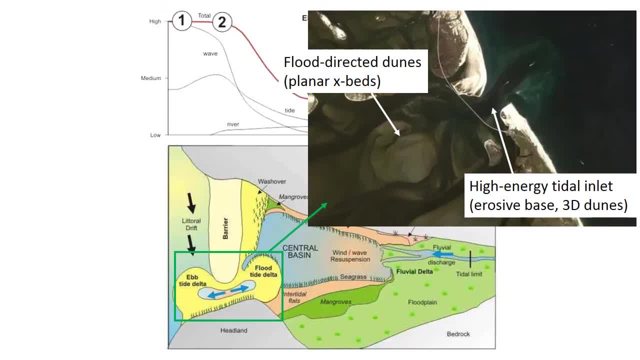 So the presence of this high-energy, tide-dominated, erosive tidal inlet is actually very significant because it can erode through older deposits as the shoreline transgresses and this creates another of these sequence stratigraphic surfaces. Note that also kind of lurking just offshore there's waves eroding the coastline. 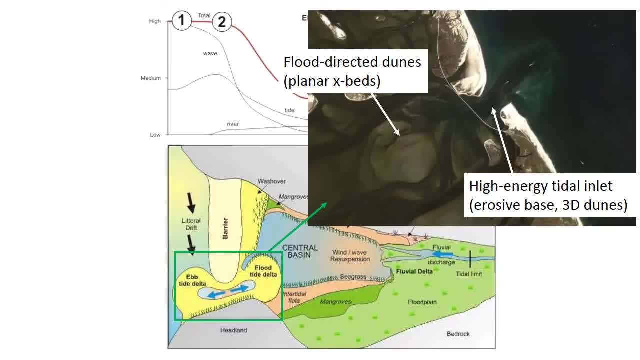 If you remember from the wave-dominated coast lecture that the shoreface profile, the profile of this coastline, is set by wave energy and wave erosion, So you can also get wave erosion from the shoreface as the whole complex transgresses over the land. 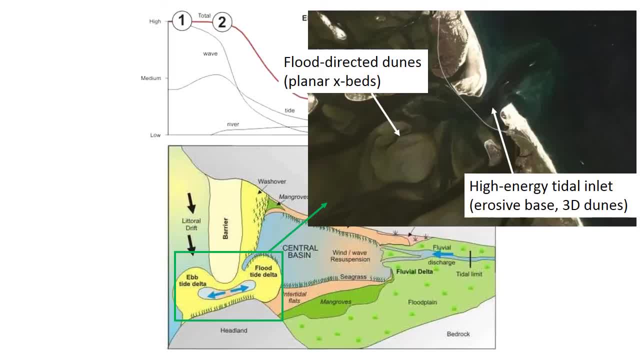 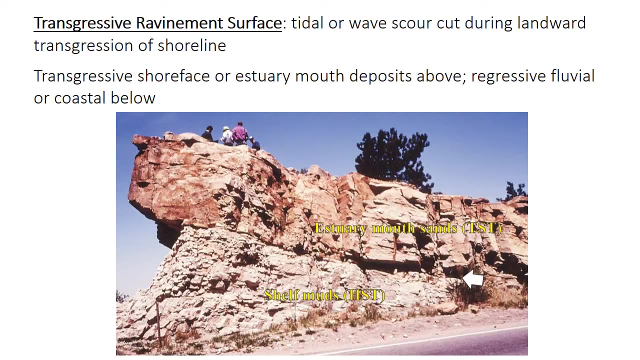 So we talked about some sequence stratigraphic surfaces before, like the regressive surface of marine erosion, the maximum flooding surface and so forth, So we'll talk about actually the final surface sequence stratigraphic surface that we haven't mentioned yet, and that is a surface called the transgressive ravinement surface. 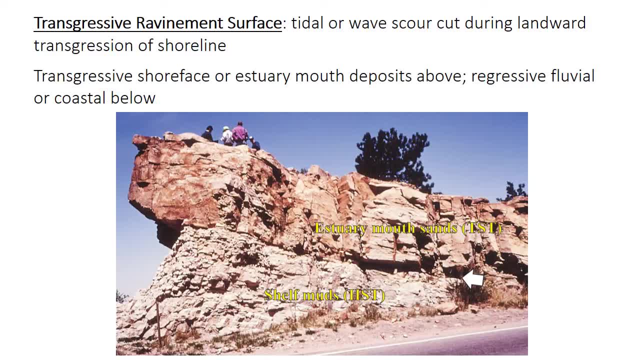 Ravinement is a word generally used to refer to erosion in a marine setting, and the surface forms due to tidal or wave scouring and erosion during transgression of the shoreline. It often forms in estuary settings because estuaries have these deep, high-energy erosive. 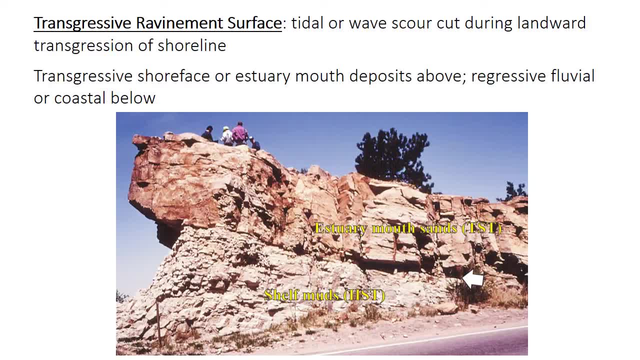 tidal inlets, but it can also form in a regular shoreface or in a barrier island. We'll discuss more next lecture. The surface is always overlain by transgressive system-strat deposits, usually shoreface deposits or estuary mouth, sort of tidal channel, tidal inlet deposits. 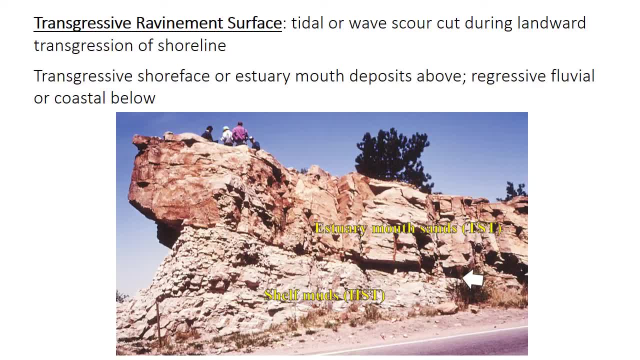 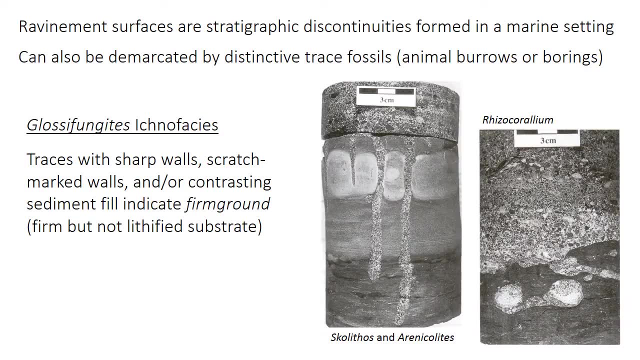 And it's underlain by regressive fluvial or coastal deposits, depending on how deeply it erodes. So ravinement surfaces form in a marine setting, so they can sometimes be recognized by a distinctive group of trace fossils. An icnofossil is a burrow or a boring made by an animal digging into the substrate. the 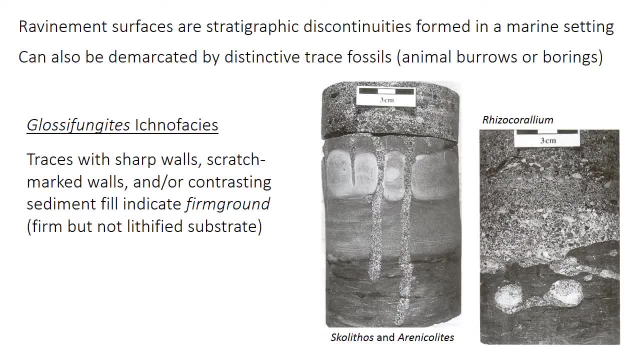 sediment. Characteristic groups of trace fossils are combined as something called an icnofaces. Like a lithofaces is all the characteristics of the rock, an icnofaces is a characteristic group of trace fossils. We'll cover icnofaces in more detail later on, but for now I just want to introduce this. 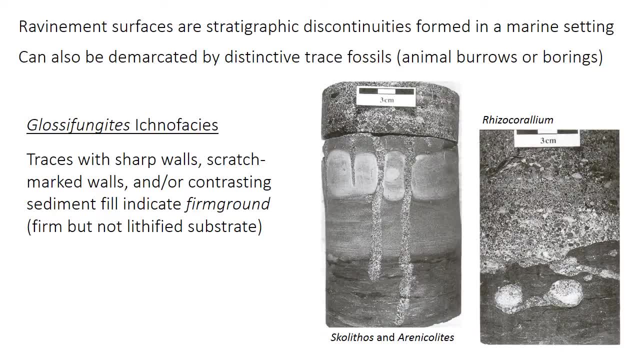 one called the glossifungides icnofaces, because it's often a good indicator of these ravinement surfaces. Trace fossils are given Latin names like scolithos or rhizocorallium. they're not important in this case. 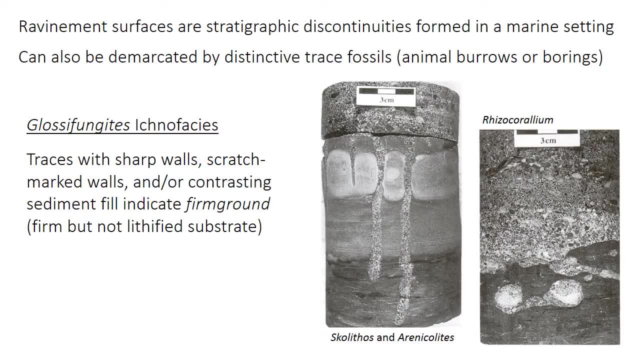 The key point with this particular type of suite of trace fossils is that they're characterized by sharp walls, a very sharp contrast between the burrow and the surrounding sediment, potentially with little scratch marks on the side of the burrow, and they often also have very contrasting 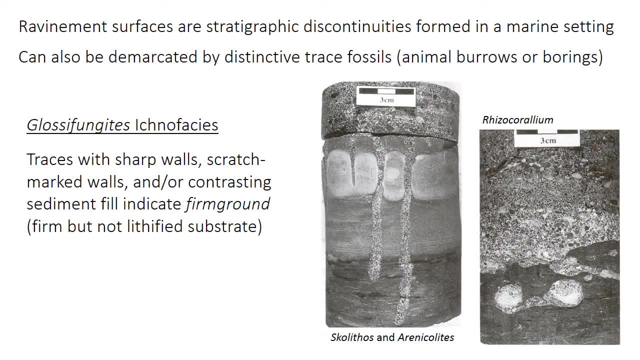 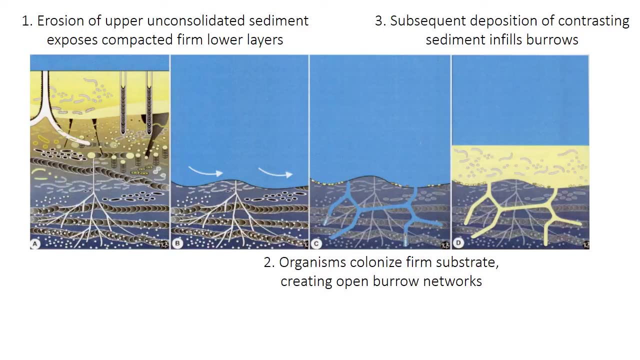 sediment fill And that's because they were dug into firm sediment. sediment that's firm, which means compacted and stiff, but it's not lithified, it's not rock, yet is often called a firm ground. So firm grounds form because ravinement erodes away the uppermost unconsolidated sediment. 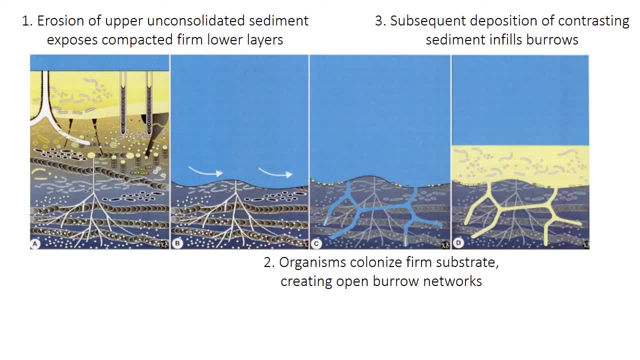 to expose underlying compacted layers. These compacted layers are firm, and so organisms will colonize that firm ground. they will dig in, create their burrows. Because the sediment's firm, the burrows will remain open after the organism dies. normally, 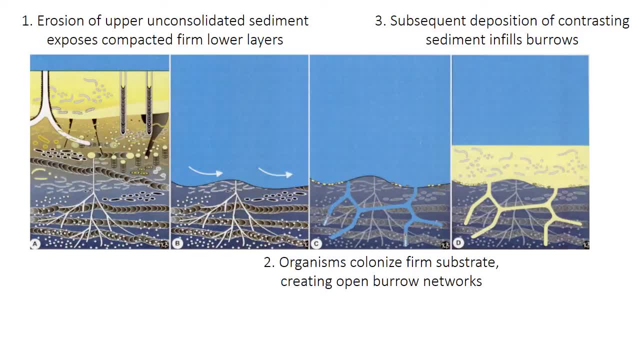 they would just collapse. They're no longer being maintained actively by the organism, And so later sediment deposition comes along and fills up these open burrows with very, very different looking sediment from what the burrows were cut into, And so this is the Glossy Fungitis ignophases. 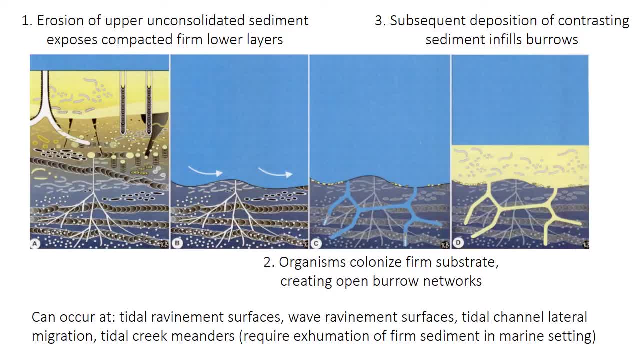 It's very typical of ravinement surfaces like the transgressive ravinement surface, but it can also occur in tidal channels, meandering tidal creeks, anywhere where you're exhuming or eroding into firm sediment in a marine setting. 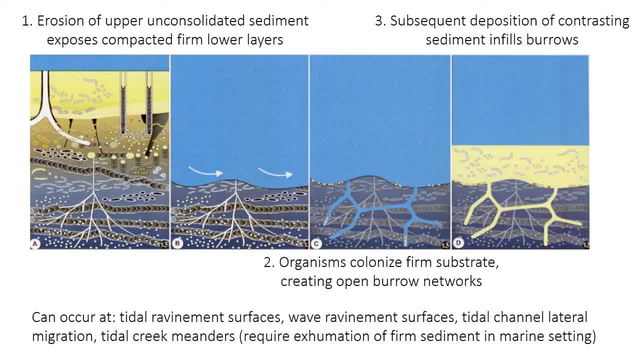 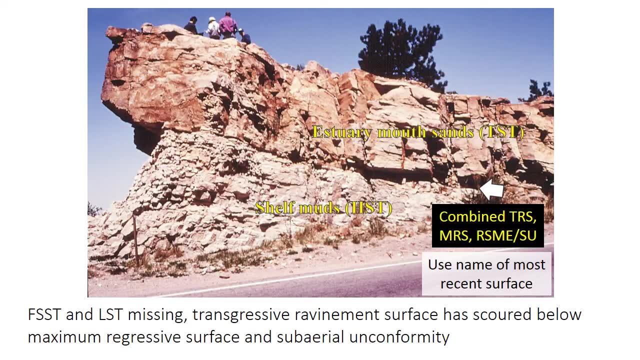 There's not that many burrowing organisms in a river, so you don't really get these sort of things in rivers. So one final point about this particular example of a transgressive ravinement surface that I showed. you know, sharp-eyed viewers might have noticed that the underlying sediments 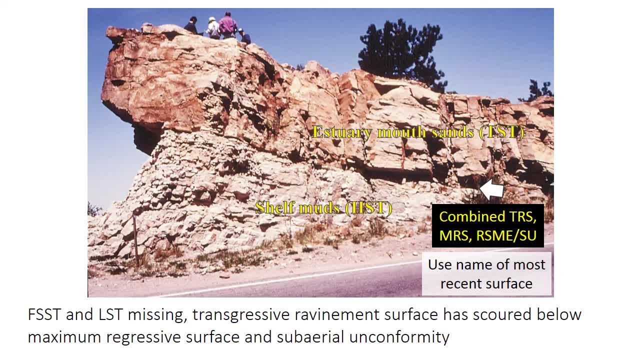 here are actually high-stand systems tract shelf sediments And that means the falling stage and the low-stand systems tracts are missing. Normally it should go high-stand falling stage, low-stand transgressive. We just go straight from high-stand to transgressive here. 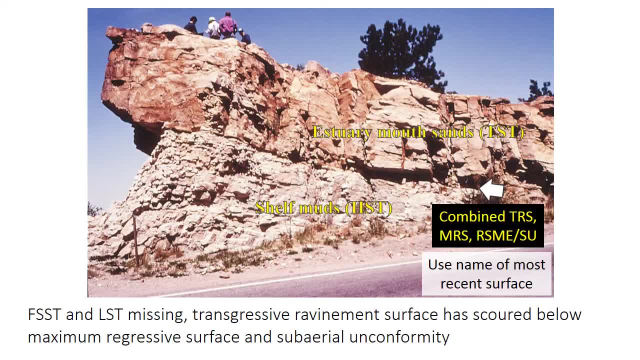 So there we go. So there presumably was a maximum regressive surface at the end of the low-stand and a subaerial inconformity or a regressive surface of marine erosion at the end of the or during the falling stage, but they're no longer present at this particular location. 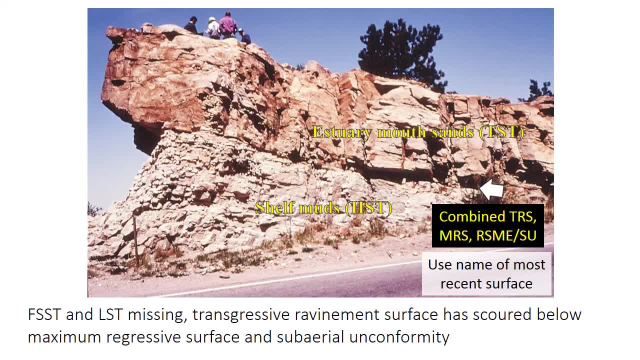 And that is likely because this ravinement surface eroded deeply all the way through and just removed them. So in cases like this, the general practice is that you use the name of the most recent surface. So in this case, because the transgressive ravinement surface is the most recent one, 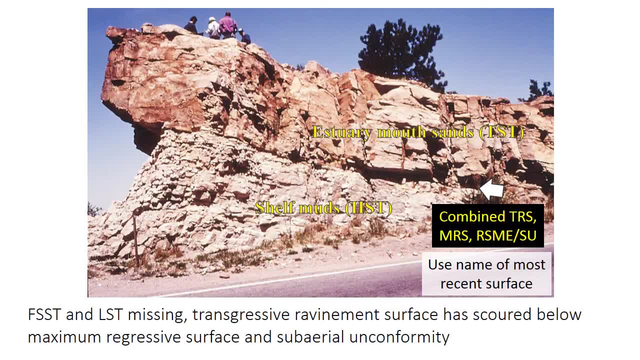 to form. That's the name that we use, So I'll just finally note that you can get ravinement surfaces that are not a sequenced stratigraphic surface. A sequenced stratigraphic surface must separate different systems tracts. It's possible to get ravinement within a systems tract, within the transgressive systems tract. 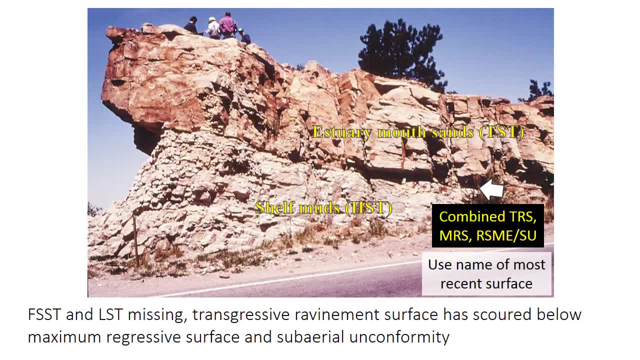 It's still a ravinement surface, but it's not the transgressive ravinement surface. It's not a sequenced stratigraphic surface. So be careful. if you see a ravinement surface, it's not necessarily a systems tract boundary. 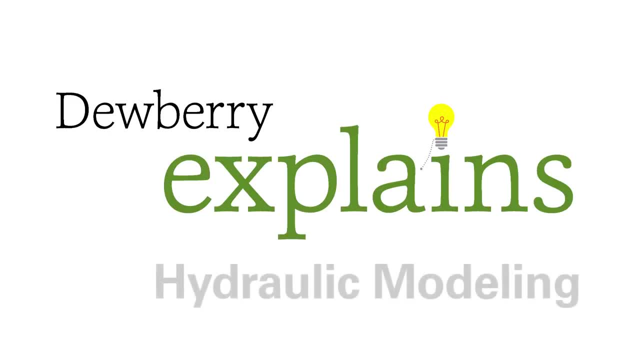 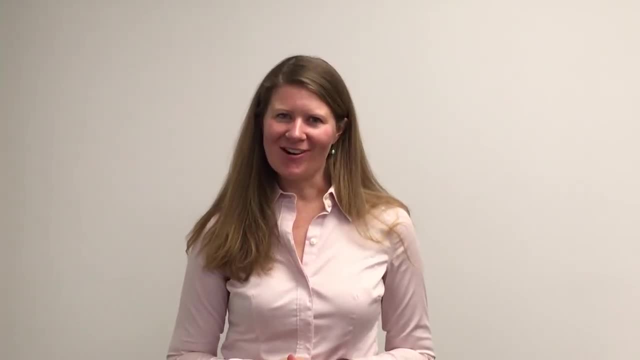 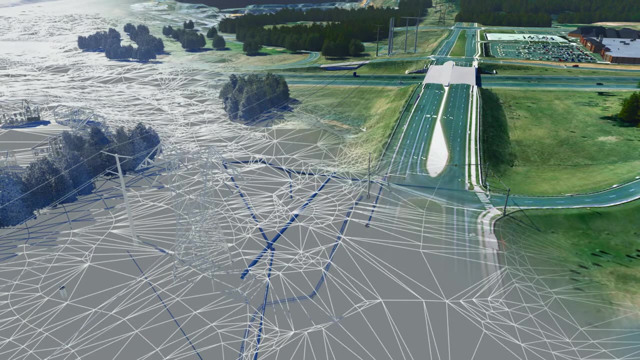 Hi, my name is Melinda Brown, I'm a professional engineer in the Denver office and I'm going to tell you a little bit about hydraulic modeling. A hydraulic model is a mathematical model of a fluid flow system, such as a water system, a sewer system or a storm system, and is 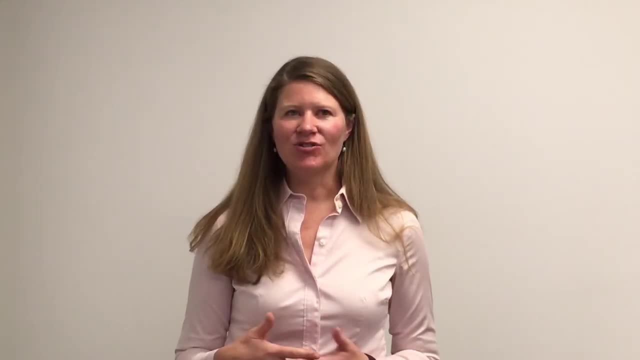 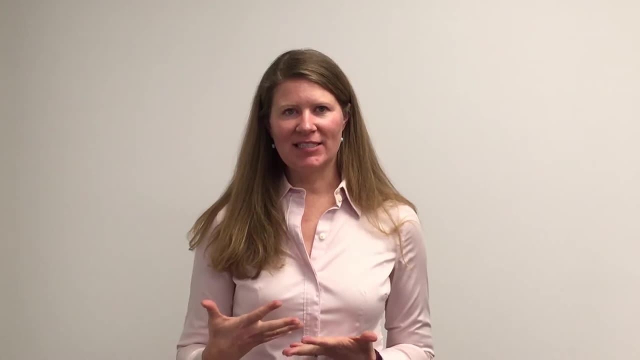 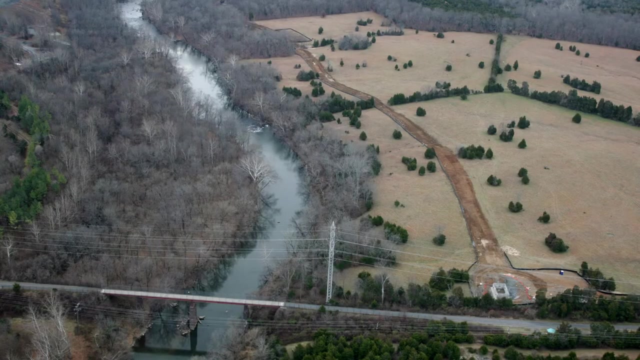 used to analyze systems' hydraulic behavior. A hydraulic model is used creating real-world data- so GIS data, CAD data or as-built pipeline system data- and you input it into the model to create a physical representation of the real-world system. You'd also use topology. 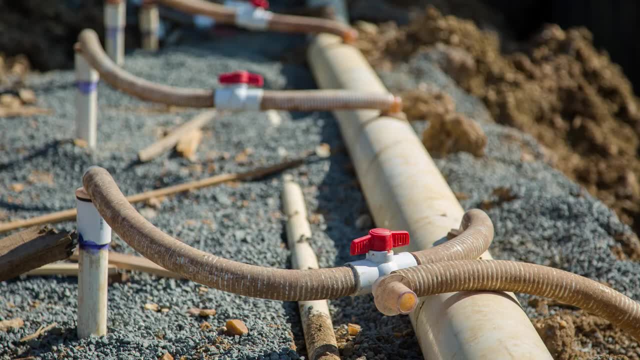 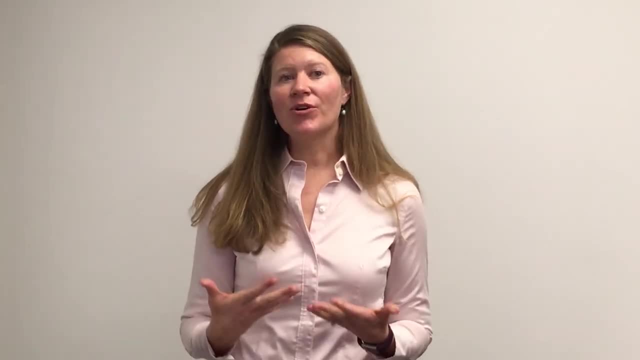 to represent the ground surface and system loading data that you would get from your client. so flow metering, water consumption records, telemetered system flows, or you could use estimates from consumer characteristics like population data, land use data or traffic.